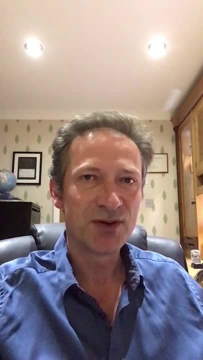 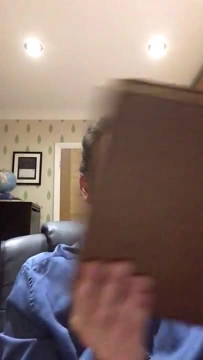 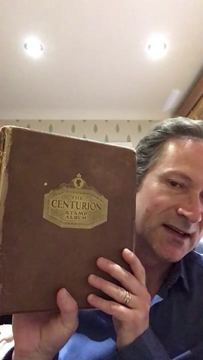 collections. So, without further ado, let me introduce the stamp collection in question, which I'm going to value for you today. And here it is. Now you can see from the front. it's an old, old Stanley Gibbons Centurion stamp album which came from the late 1930s. So we suggest. 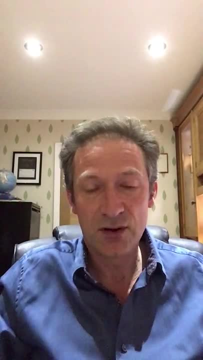 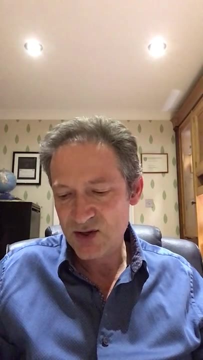 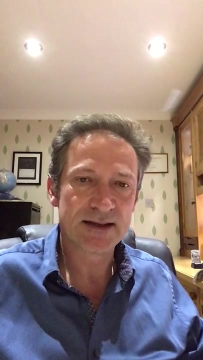 there's some old stamps in here Could have some value. but let's have a look. So opening up. Oh so at the front of the album the collectors dated it 17 Jan 1962, total stamps in the album: 1173.. So what this looks like is a typical boyhood stamp collection from the 1960s. 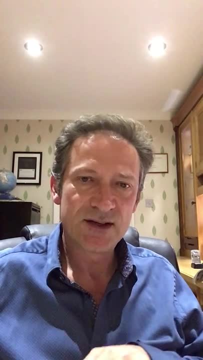 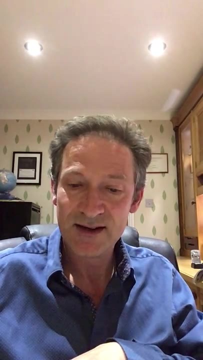 which is a typical boyhood stamp collection from the 1960s, Which is not in keeping with the age of the album, which suggests to me that this person's father collected and handed this collection down to his son. So what I would expect to find is that all. 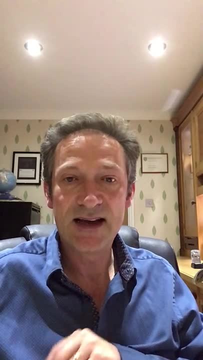 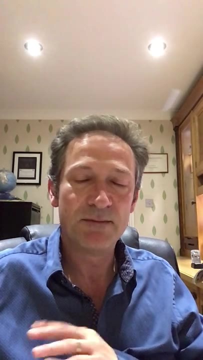 the stamps in here that the collector in question has added from the 60s and 70s will have very little value, And the reason for that is that millions were printed at that time and very few have value. So it's really going to be all about. 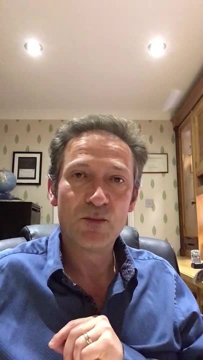 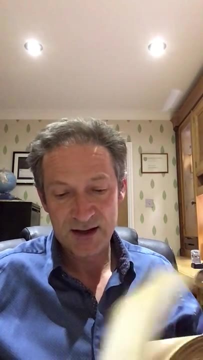 the older stamps that his father put into the album. But the most important thing now is to have a look at the condition of the stamp. So I do that just by having a very, very quick flick through pages and you can very quickly see what the condition is like. Okay, right, So I can tell. 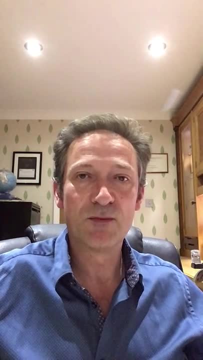 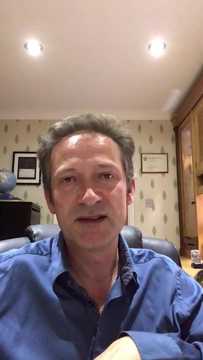 straight from that that the condition is poor. They're like typical boyhood stamp collections. They're all stuck to the pages. It looks like the majority is modern from the 60s and 70s, but there are some old stamps that clearly. 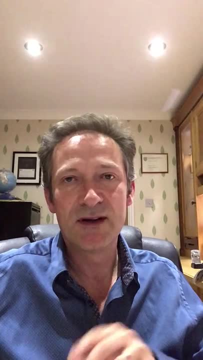 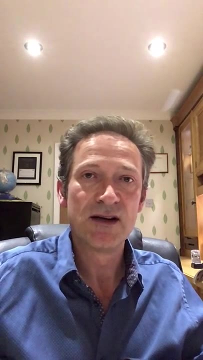 the collector's father put in The mint stamp stuck in will be worth a fraction of the catalogue value, unfortunately, and it will really be all about whether there's any rarities in here which I would at this stage suspect to be unlikely. I'll give you an example of a page. 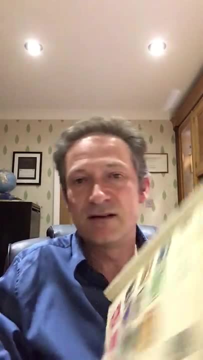 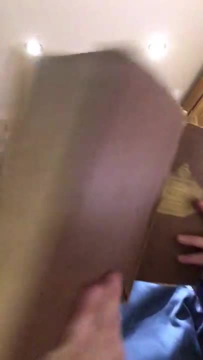 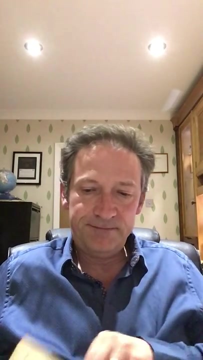 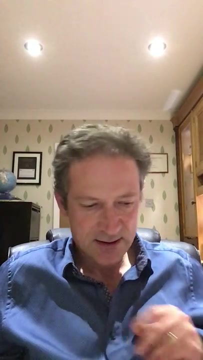 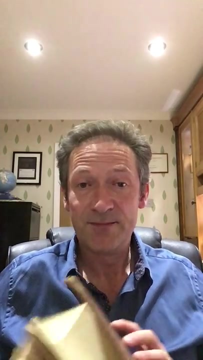 to give you an idea of what the condition looks like, Here's Belgium, As you can see, not good condition and mainly modern. So let's look at Great Britain And see if we can find anything of value there, Right? So, as I suspected, it's not of value. There are some old stamps in here, but the condition is: 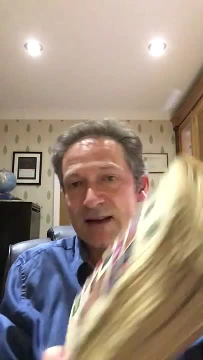 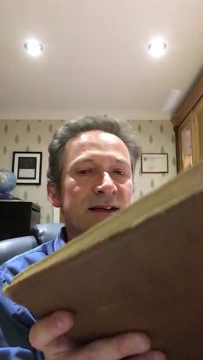 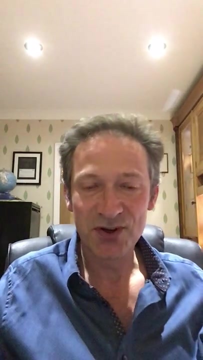 terrible and they're not particularly rare: old stamps. Here's an example page for you, Interesting But of very little value. So unfortunately, mainly because of condition stamps falling out of it, which gives you an idea what the condition is like. 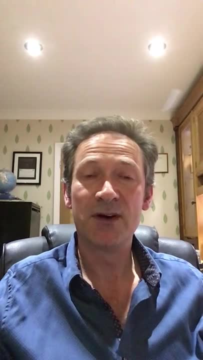 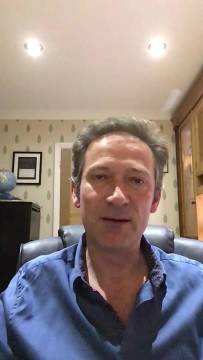 I would value this collection at around about £500, which might even be generous. What I would actually say is it's a really interesting stamp album with old maps in it, and it's an actual very nice collection. We've given a good sort of range of stamps. 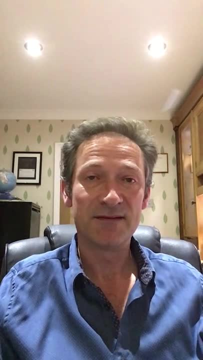 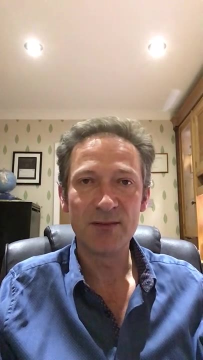 and I would suggest that keep it in the family as a family heirloom. I think it has more personal value than monetary value and it will rise in value over time, despite its condition. I think just from doing this gives you an idea what life's like for us, because we only trade in. 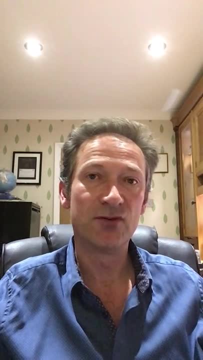 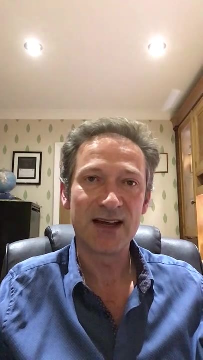 that 0.1 percent. so we have to kiss a lot of frogs to meet our print And all we sell is top quality, rare stamps and it's a very challenging thing to do. So I mean, if you think about it, you can certainly see that this is a really good stamp. 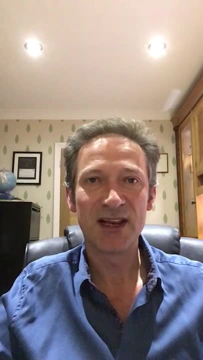 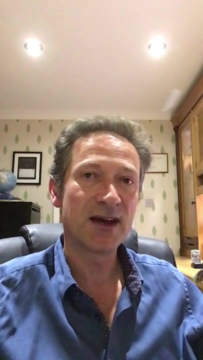 If you think you are in this 0.1% and you have a collection that you think is of value and you're interested in a valuation with a view to selling, please get in touch with me at mike at justcollectingcom. Rest assured: collections with value take. 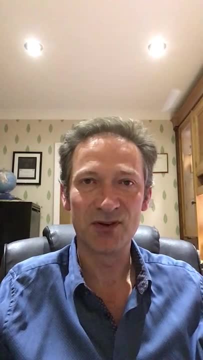 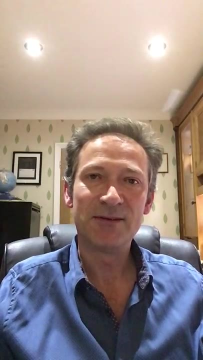 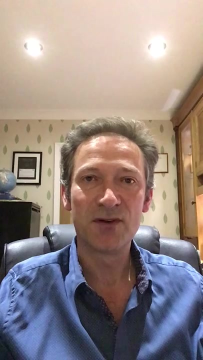 considerably more time than it does for the vast majority of collections, which are, in fact, boyhood collections of little value. I think that's all for today. Good to speak to you. I hope that you found this informative and I look forward to speaking to you again next week. Thank you very much. Goodbye.